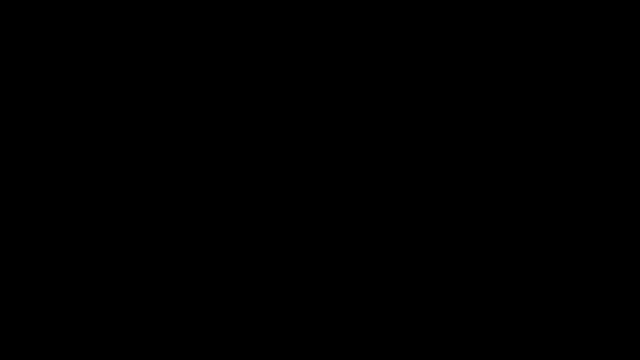 Now, sometimes you may need to divide by two numbers. Let's say, if we want to divide 9 factorial by 7 factorial, What's the best way to do this? 9 factorial is 9 times 8 times 7 times, 6 times, 5 times 4, all the way to 1.. 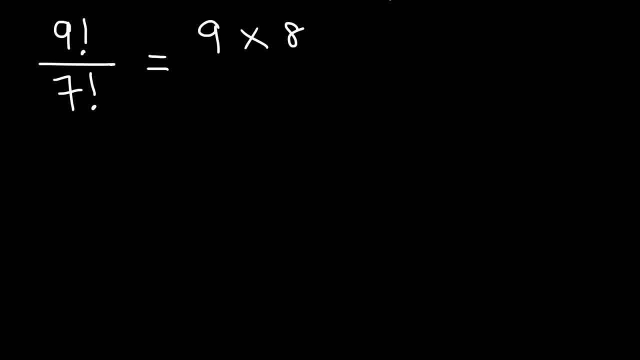 Well, instead of writing 7 all the way to 1,, 7 times, 6 times, 5 times, 4 times, 3 times, 2 times 1.. All of that is simply 7 factorial, And it's best to write it that way. 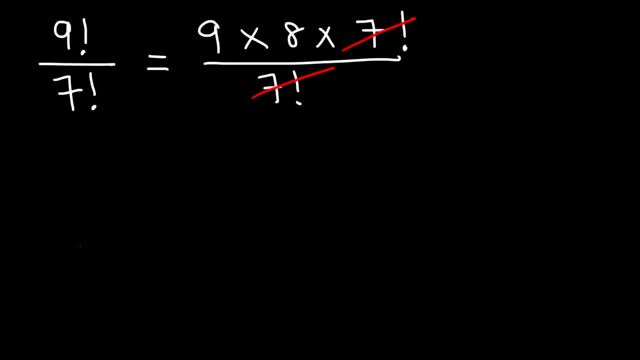 Because notice that we can, And so if we do it that way, there's a lot less writing And therefore it's just 9 times 8, which is 72.. So that's 9 factorial divided by 7 factorial. Let's work on another similar example. 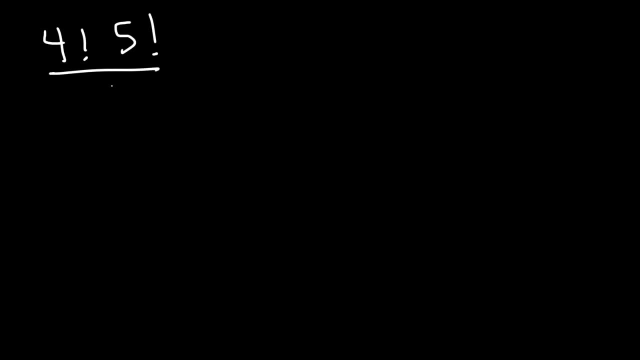 So 4 factorial times 5 factorial, divided by 6 factorial. Go ahead and simplify Now: 4 factorial is 4 times 3 times 2 times 1. And 5 factorial. I'm going to leave it the way it is. 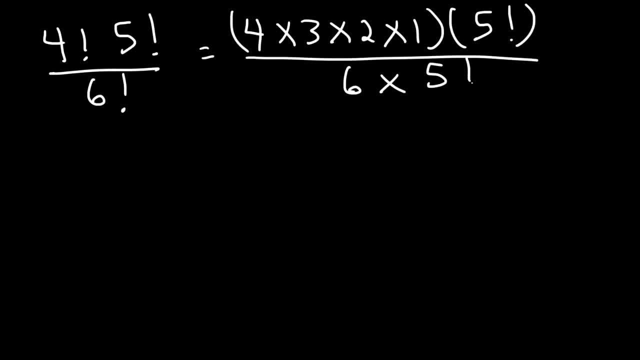 6 factorial is 6 times 5 factorial, So I can cancel 5 factorial. Now the 1, 1 is not going to change anything, so I can drop that. So I have 4 times 3 times 2.. 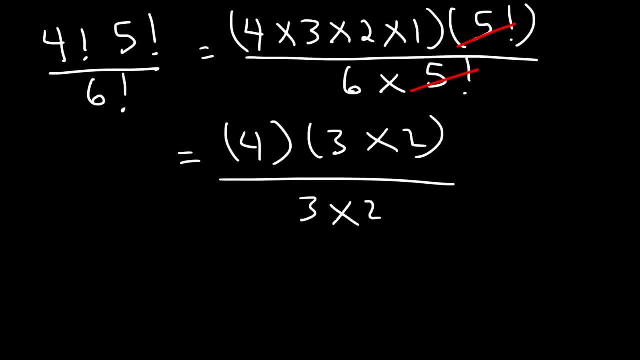 And 6, I can write that as 3 times 2. Which can be cancelled. So the final answer is 4.. Now, what is 0 factorial? What is that equal to 0 factorial, if you ever see it is 1.. 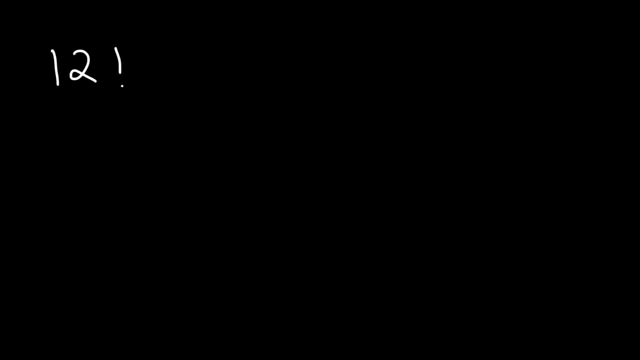 So just keep that in mind. Try this one: 12 factorial divided by 3 factorial, That's going to be 3 times 2 times 1.. Now 12 factorial, that's going to be 12 times 11, and then times 10 factorial. 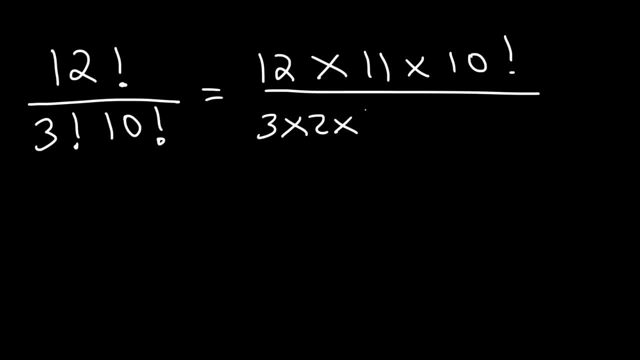 3 factorial is going to be 3 times 2 times 1.. And let's cancel 10 factorial. Now, 3 times 2 is 6.. And 12 divided by 6. That's going to be 2.. So we got 2 times 11.. 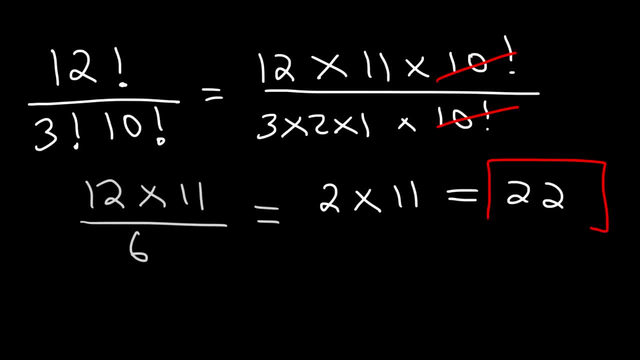 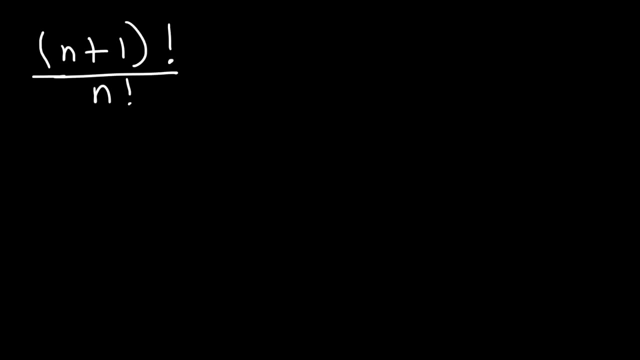 And so the final answer is just 22.. And that's it. Now, sometimes you might be given an algebraic expression with variables as opposed to real numbers. So let's say, if you want to simplify the expression, n plus 1 factorial divided by n factorial. 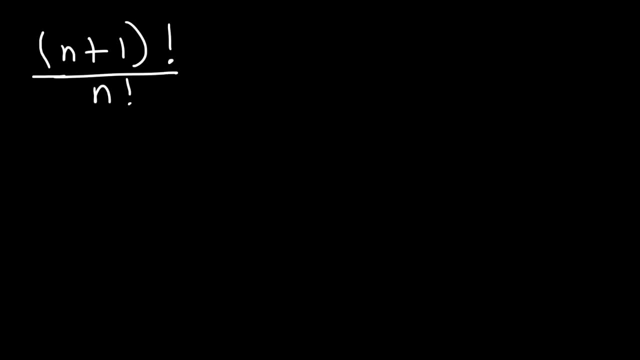 How would you go about doing it? Now? let's say if n was 7. And you want to simplify the expression, That means we would have 7 on the bottom and n plus 1 would be 7 plus 1, or 8 plus. 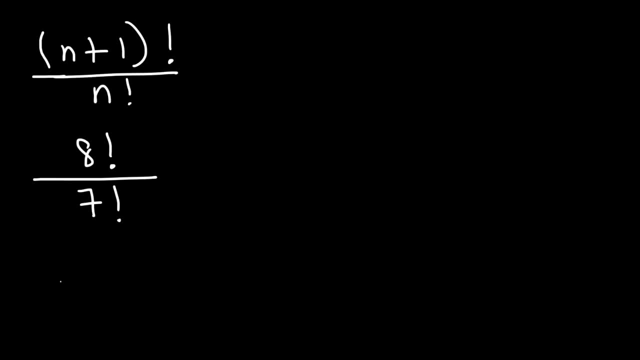 1. What would this simplify to? Now, let's say if we had, if n was 10. That means n plus 1 would be 11. What would 11 factorial over 10 factorial simplify to? Let's see if there's a pattern. 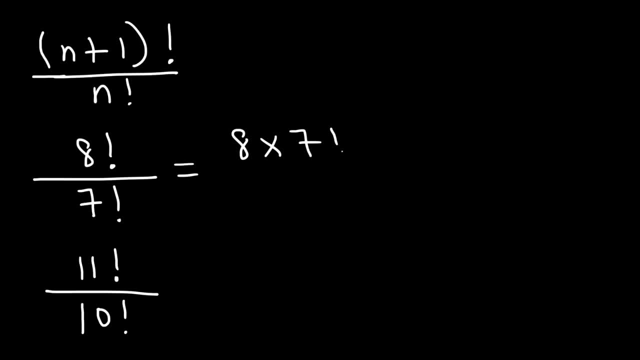 So 8 factorial is simply 8 times 7 factorial, And so we could cancel 7 factorial. So 8 factorial is simply 8 times 7 factorial. So when you are writing out factorial, the next number is always going to be one less. 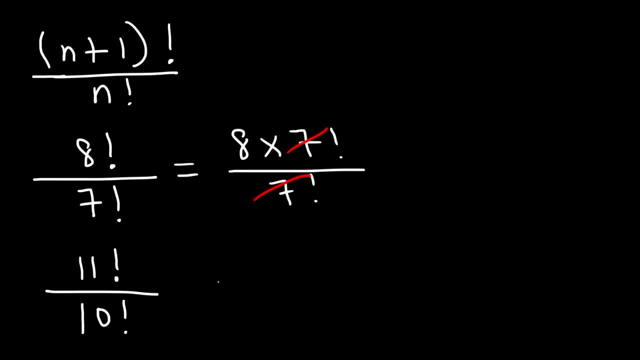 than the previous number. So for 11, factorial it's going to be 11, and then 1 minus 11, or rather 11 minus 1.. That's going to be 10.. So that's the next number in the sequence. 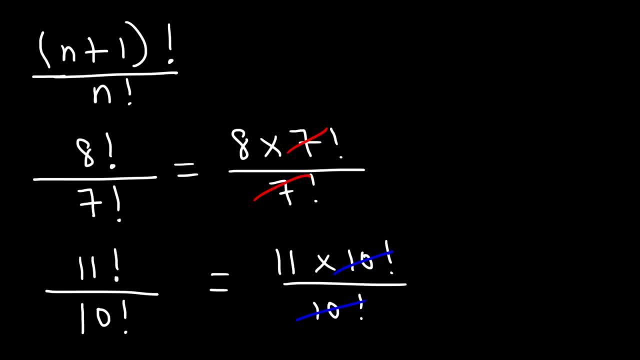 And so we could cancel 10 factorial. So 8 factorial over 7 factorial is just 8.. 11 factorial is just 8.. 8 factorial is just 8.. over 10 factorial is simply 11.. So it turns out that it's equal to whatever this number is. 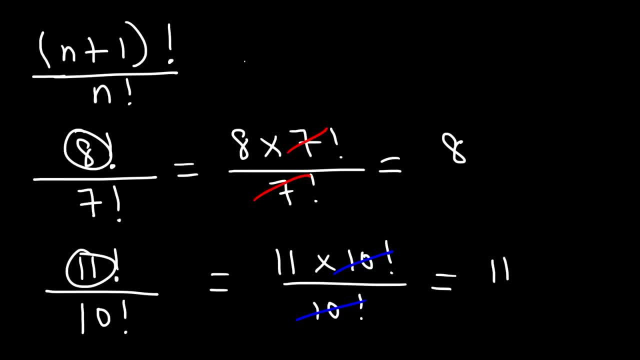 And that number is n plus 1.. So this should simplify to n plus 1.. But now let's see if we can get that same answer algebraically. So n plus 1 factorial, that's going to be n plus 1.. 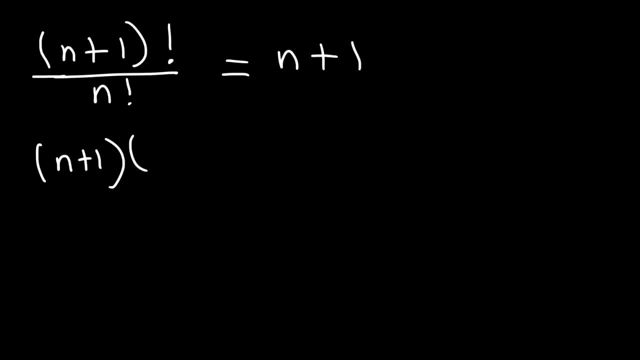 And then 1 less than n plus 1 is n. 1 less than n is n minus 1.. And it's just going to keep on going. Now n factorial is going to be n, and then 1 less than that is n minus 1.. 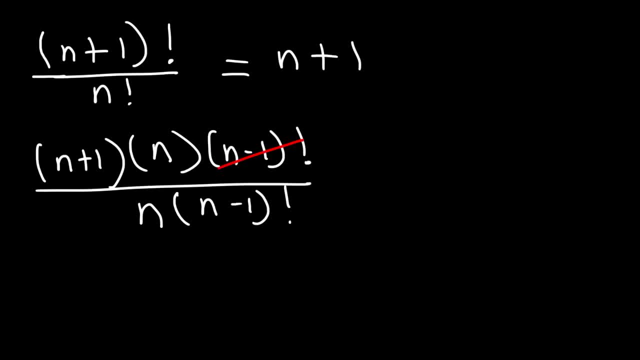 And that's going to keep going. So we can cancel n minus 1, and we can cancel n, And so we're going to be left over with simply n plus 1.. And that's the answer. Here's another one that you could try. 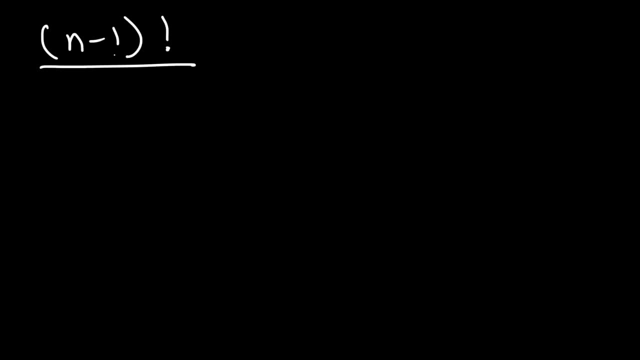 n minus 1 factorial divided by n factorial. What does that simplify? to Now, n minus 1 factorial is less than n factorial. So I'm going to rewrite it like that, Or we can take the next one: 1 less than n minus 1 is. 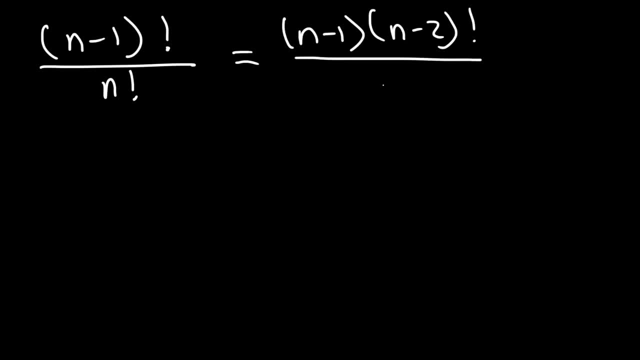 n minus 2.. n factorial is going to be n, and then 1 less than that is n minus 1.. And 1 less than that is n minus 2.. So we could cancel n minus 2 factorial and we could cancel n minus 1.. 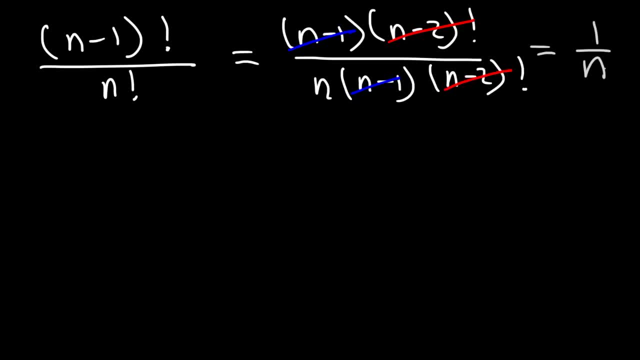 So therefore, the answer is going to be 1 divided by n. Now let's illustrate it with some examples. So let's say: If n is 8, that means n minus 1, or 8 minus 1 has to be 7.. 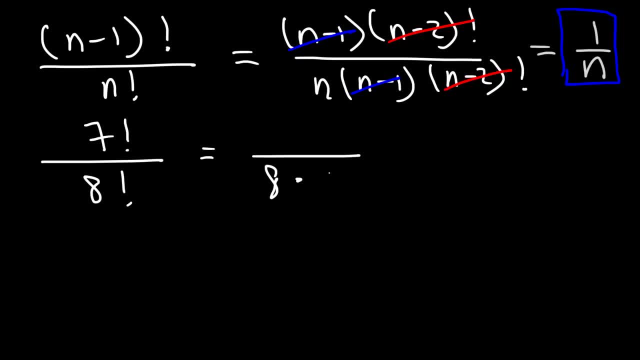 So 8 factorial is going to be 8 times 7 factorial, And we could cancel 7 factorial And so we get 1 over 8.. So since 8 is n notice that we get 1 over n, Try this one. 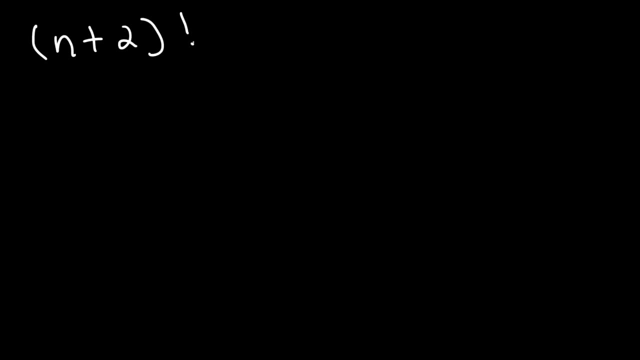 n plus 2 factorial divided by n factorial, So n plus 2 is the larger number in this case. So it's going to be n plus 2.. And then 1 less than that is going to be n plus 1.. And then if you subtract that by 1, you get n.